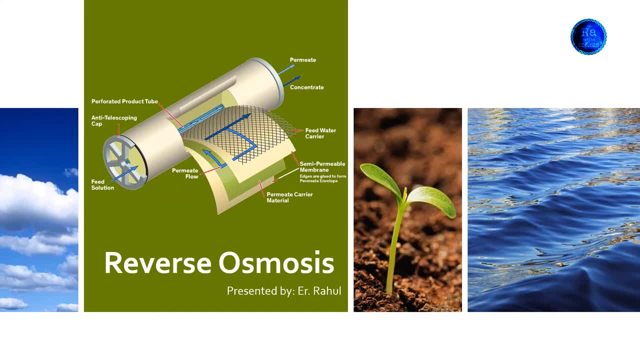 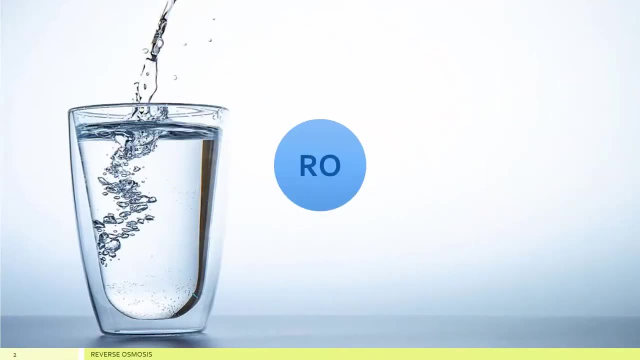 Hi, this is Rahul, and in this video I am talking about reverse osmosis, Why ROE is important, why this process implemented for desalination of wastewater. So let's start this presentation. In this video I am discussing about the introduction and concepts. What are the basics in ROE process? ROE is completely safe and healthy to consume and one of the best options in today's environment. 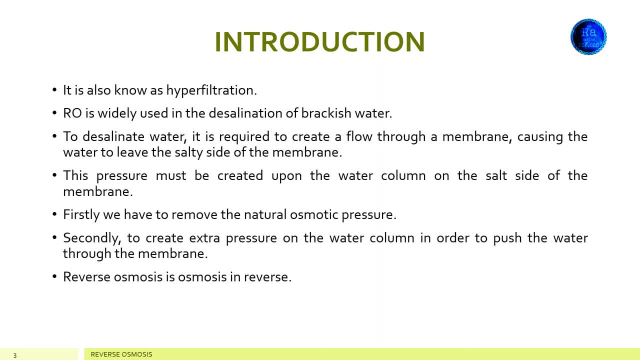 ROE is less harmful to the environment. ROE is less harmful to the environment. ROE, as commonly known as hyperfiltration, is a high-pressure, energy-efficient technique for developing for dewatering process streams, concentrating low-molecular weight substances in solution or purifying wastewater. It has the ability to concentration dissolved as well as suspended solids. ROE is widely used in the desalination of brackish water. 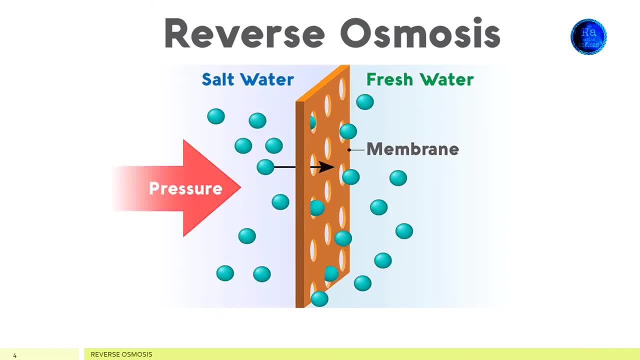 To desalinate water, it is required to create a flow through a membrane, causing the water to leave the salty side of the membrane, passing upon the water column on the salt side. To achieve this, pressure must be created upon the water column on the salt side of the membrane, firstly to remove the natural osmotic pressure and second on is to create extra pressure on the water column and salt side. 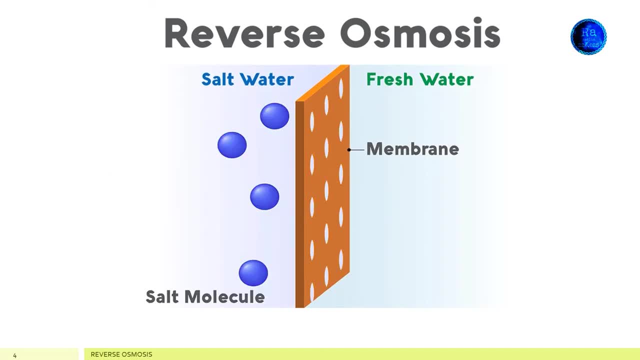 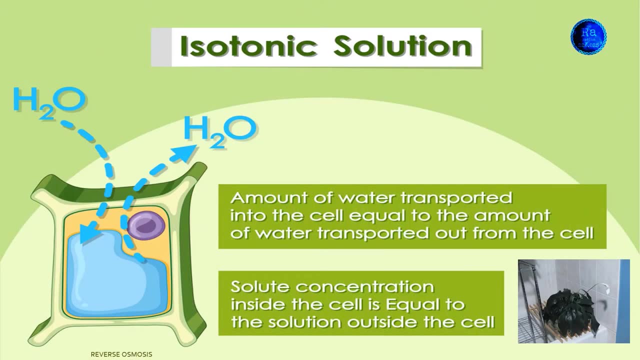 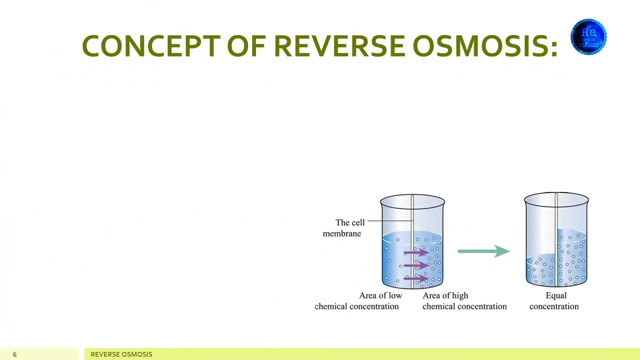 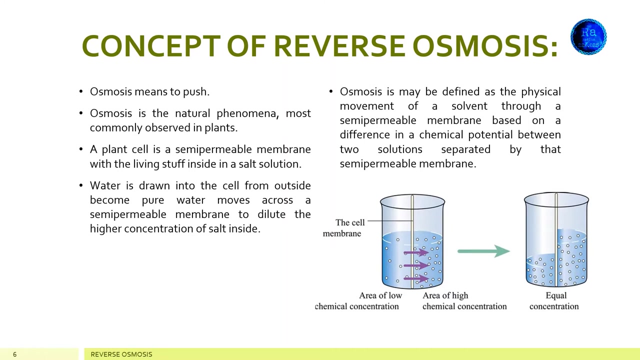 What is osmosis? Osmosis is the natural phenomena most commonly observed in plants. Osmosis is the natural phenomena most commonly observed in plants. What is osmosis? Osmosis is the natural phenomena most commonly observed in plants. What is osmosis? Osmosis is montón d'いつ grindingности. I call the heavens or theiony. Ossynos, synax, havers, spite, weed spray, thorny salt, haversλεiness, partiselaARE. you slowly petered off. challenge: asset equation. 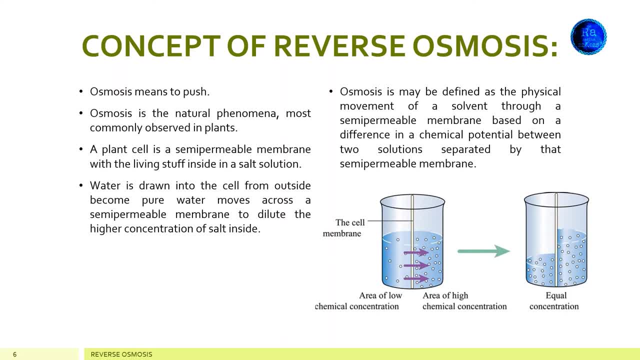 a plant cell is a semi-permeable membrane with the living stuff inside. in a salt solution, water is drawn into the cell from outside. become pure, water moves across a semi-permeable membrane to dilute the higher concentration of salt inside. osmosis may be defined as the physical movement of a solvent through a semi-permeable membrane.